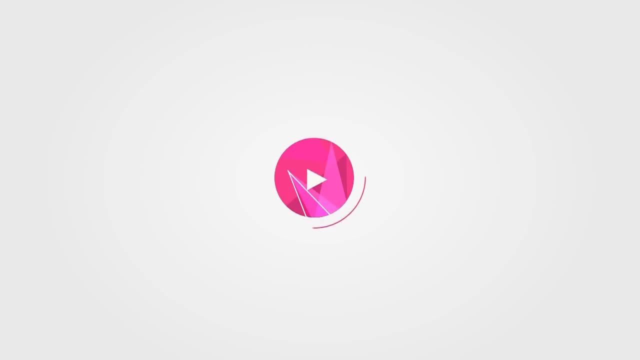 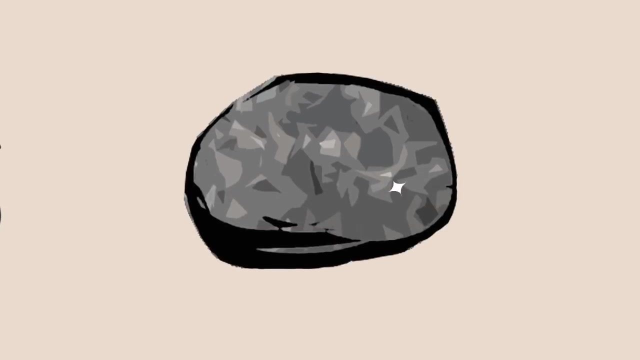 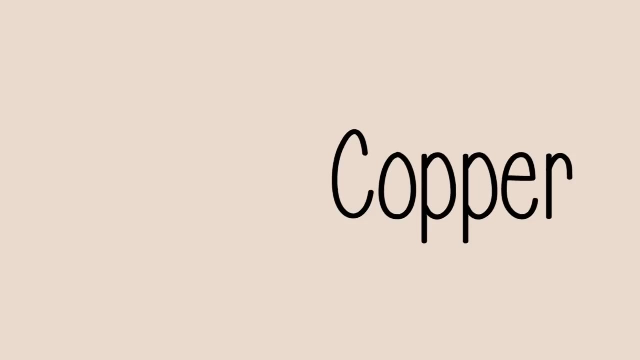 Certain metals can be extracted from their ores. For example, iron is extracted from hematite in a blast furnace and copper can be extracted from malachite. The process of extracting metals from their ores can be time-consuming, costly and harmful to the 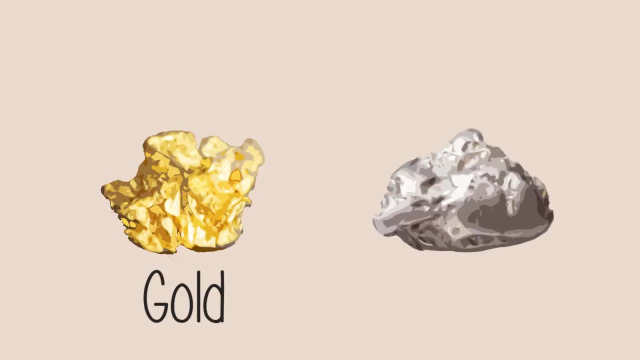 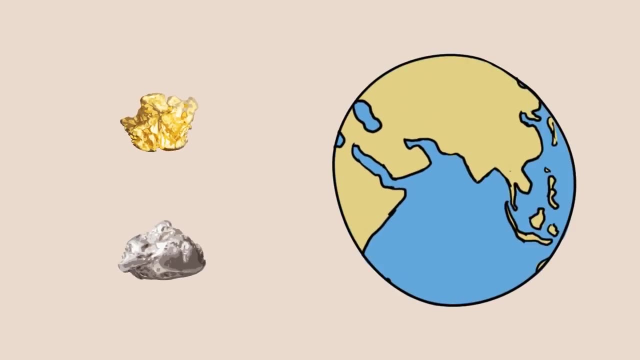 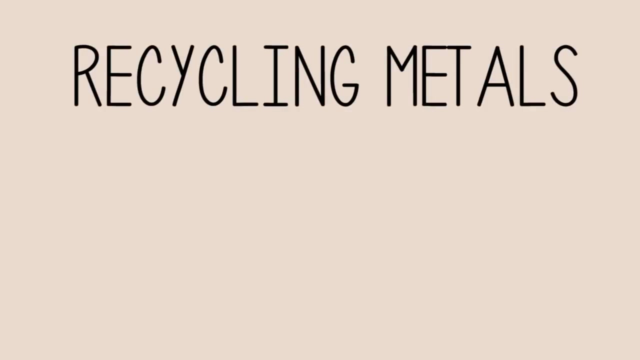 environment. Other, less reactive metals, such as gold and platinum, can be found naturally as native metal. The issue here is that there is a finite or limited supply of these metals on Earth. In this lesson, we will learn about recycling metals and the advantages and disadvantages. 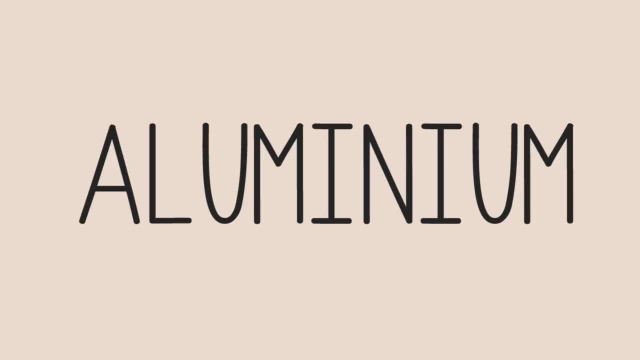 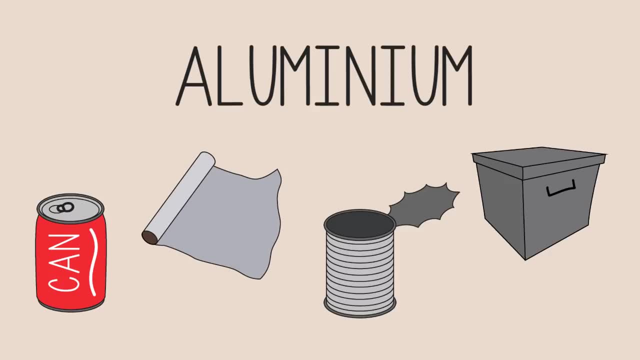 to these industrial processes. Aluminum is the most commonly recycled metal. Aluminum is used to make soft drink cans, aluminum foil, certain food cans and even certain packaging materials. Aluminum is also used to make the outer bodies of some cars and airplanes, due to the fact that it 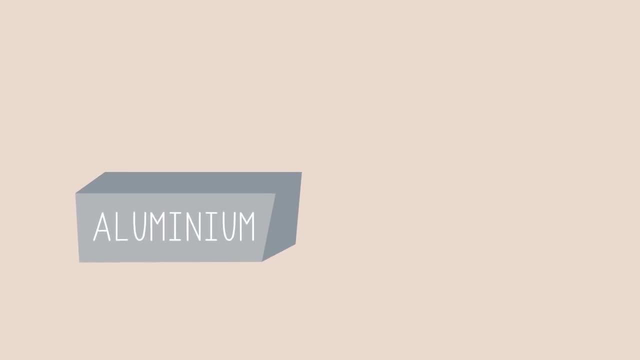 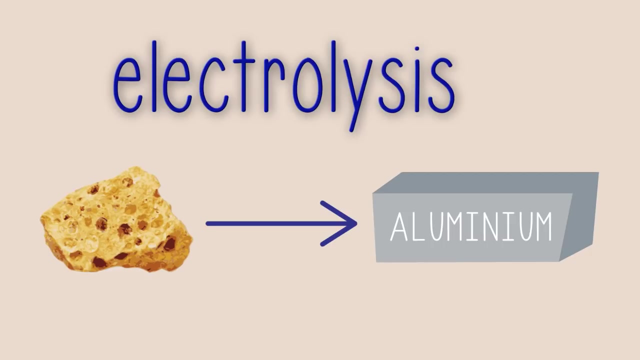 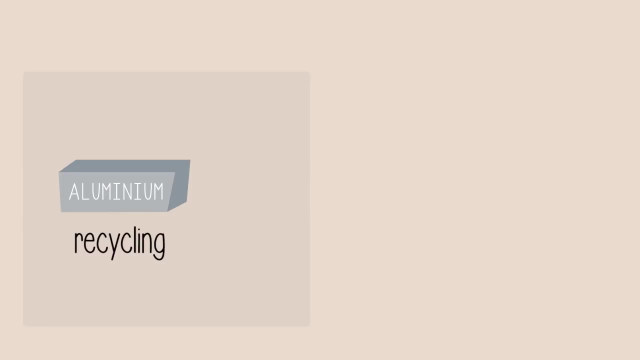 is less dense than steel. The extraction of aluminum from its ore is done by electrolysis. It may not seem like a lot of electrical energy is needed, but keep in mind that this is done on an industrial scale. worldwide, The recycling of aluminum uses only 5% of the energy used in. 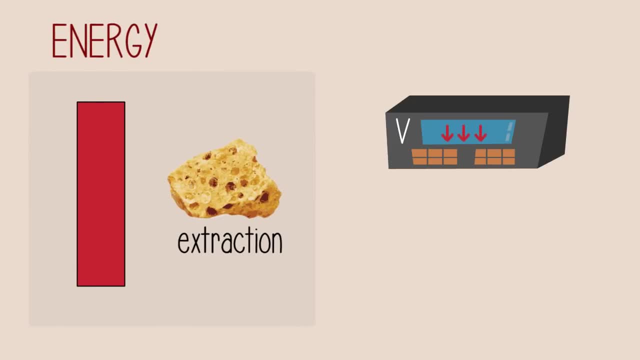 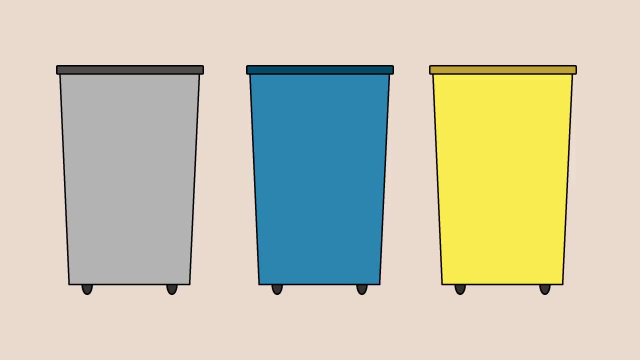 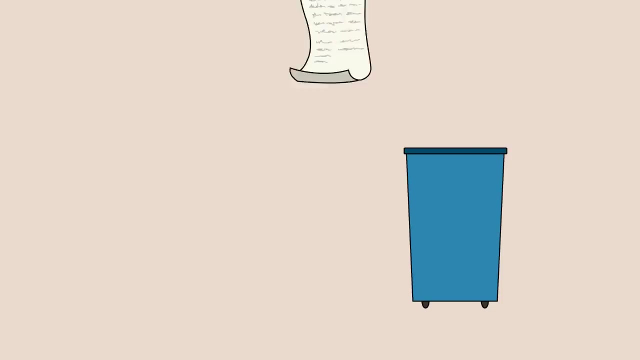 its extraction from its ore, which uses a small voltage but a large current. In fact, some countries really encourage recycling by having separate sections in their public waste containers: one for waste, one for cans, one for other metal products and another for paper products. Some countries also have mandatory 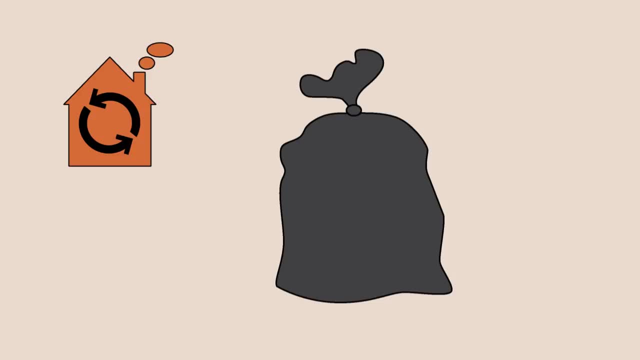 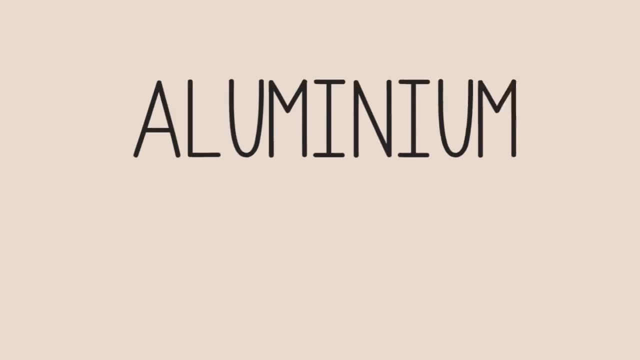 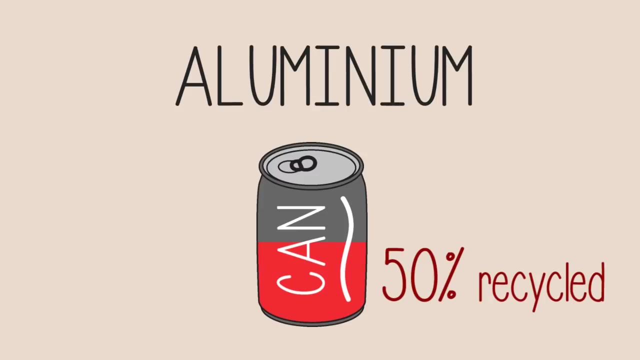 household recycling in a sense that if aluminum cans are found in regular waste bins for pickup, a fine can be issued. In fact, recycling aluminum is so common that any aluminum material that you encounter today has some, if not more than 50%, recycled aluminum content. Steel can be recycled. 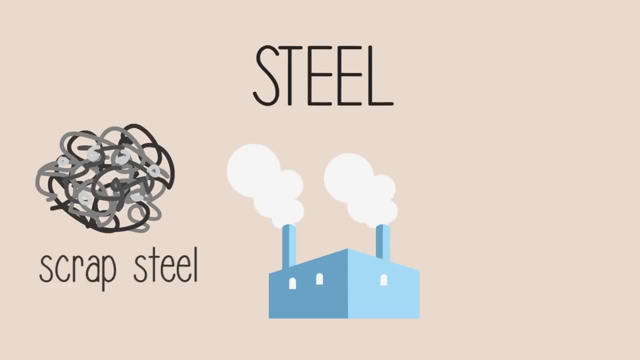 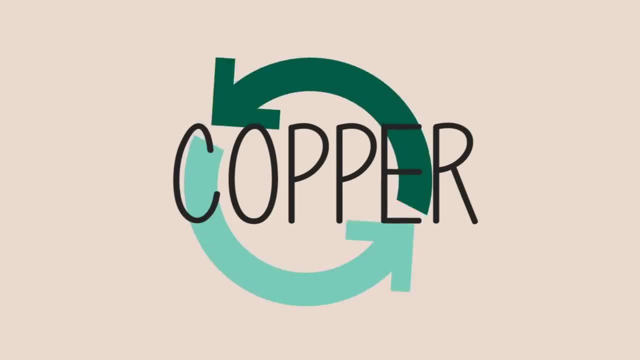 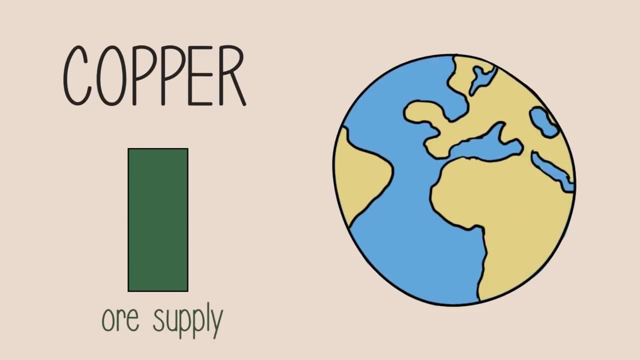 and most steel mills, particularly steel mills, are made of aluminum. Aluminum can be recycled. primarily, use recycled scrap steel instead of cast or pig iron from blast furnaces. Copper is also recycled. Once again, this is a more energy-efficient process than the extraction from its ore As well. the copper ore supply on Earth is being depleted at a very fast rate. 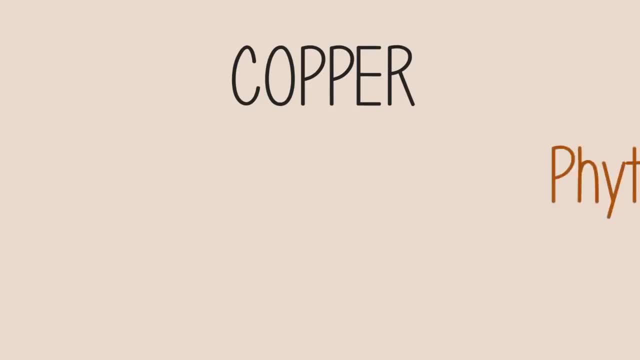 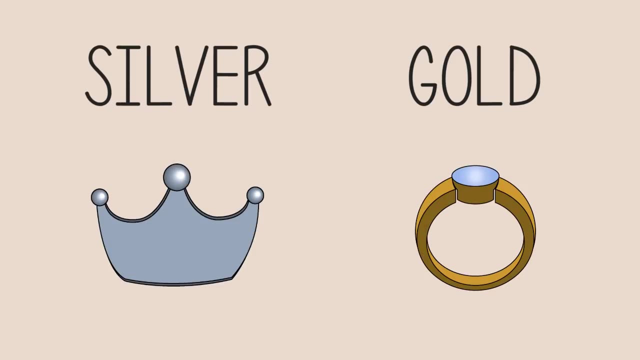 As a result, other methods for the extraction of copper, such as phytomining and bioleaching, are being used instead. Gold from jewelry are also recycled, As these metals are found as native metals. the issue here is not the energy cost, but rather the rarity of these metals. 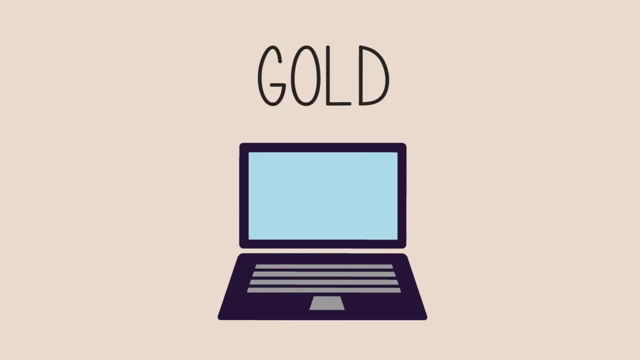 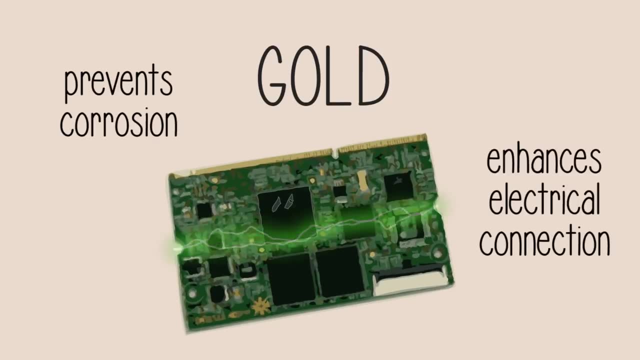 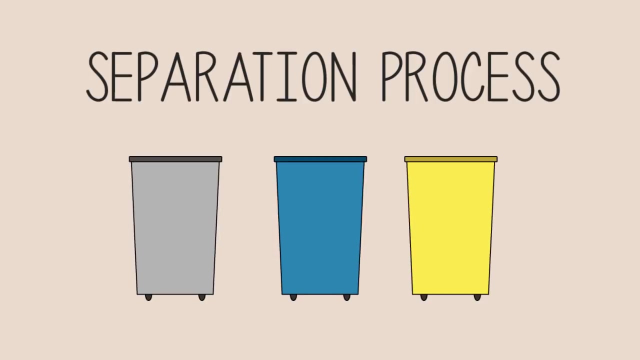 The main source of gold is recycled electronic goods such as computers, which have their electrical contacts plated with gold, so there is no corrosion and a perfect electrical connection. The main issue with recycling metals is the separation process in the waste containers, most often in the waste containers and most often in the waste containers. 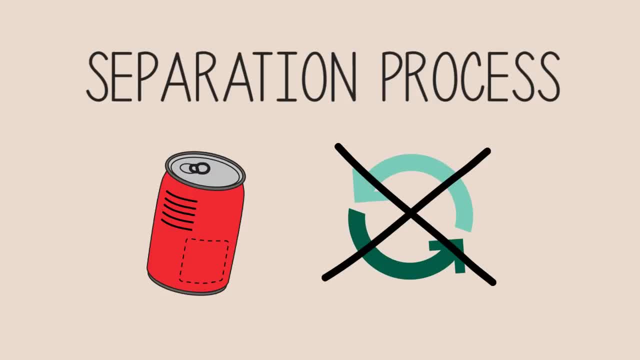 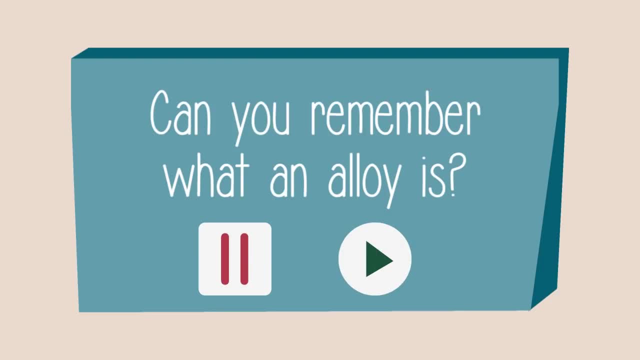 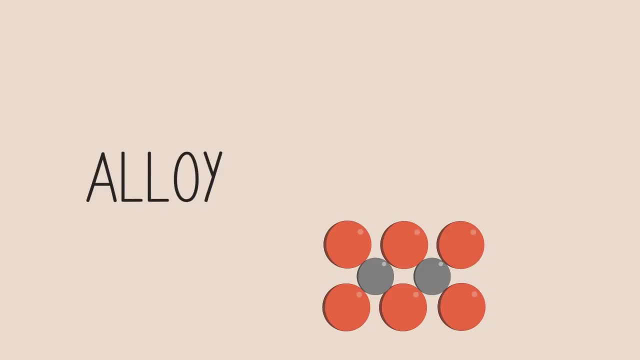 In addition, not all metal products are clearly labeled as recyclable As well. many metal products are alloys. Can you remember what an alloy is? Please pause the lesson and continue when you are ready. An alloy is a mixture of two or more elements, with at least one of the elements in the mixture 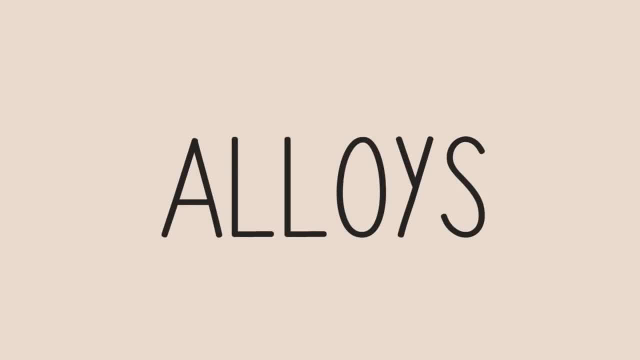 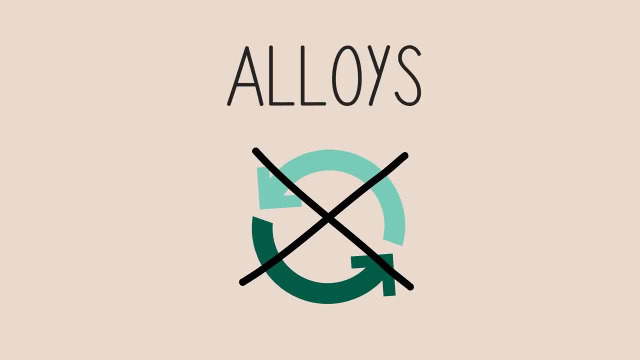 as a metal. Many metal products are made into alloys for increased strength and other desirable properties, but not all alloys can be recycled. In addition, not all metal products are recycled. Some alloys which can be recycled need to be molten and separated into their constituent metals. thereby making it a more energy-costly process As well. we have to take into consideration the fact that these metal products must first be collected and then transported to recycling facilities, All depending on the distances covered. this could involve quite a bit of fuel usage. The reason for this is that all metal products are recycled in the same way. The reason for this is that all metal products are recycled in the same way. The reason for this is that all metal products are recycled in the same way. In summary, aluminum, steel and copper are the most commonly recycled metals. 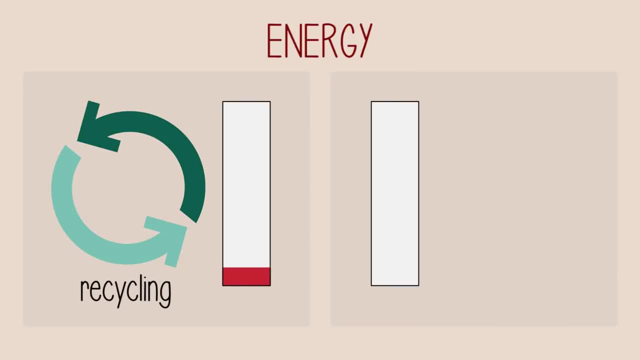 and the recycling process usually uses significantly less energy than extraction from their ores.